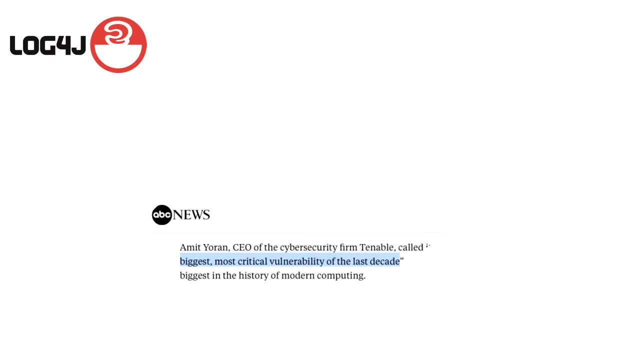 earlier is the recent log4j, which Tenable referred to as the single biggest and most critical vulnerability of the last decade. Log4j, or log4shell, might be the worst exploit that we have ever seen, due to several factors, including how easy it is to execute and the 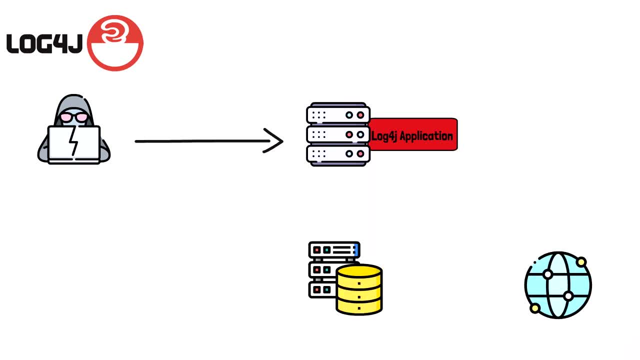 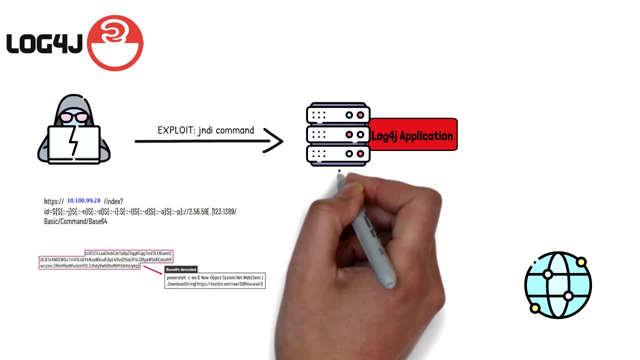 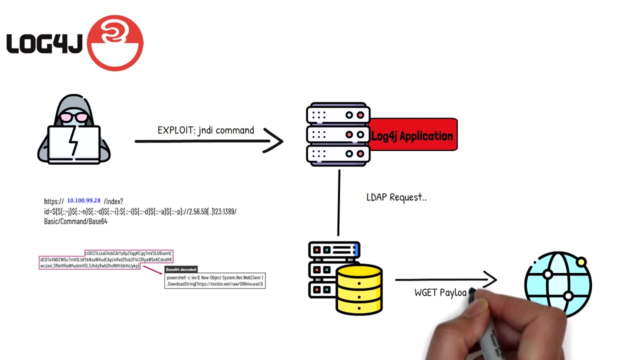 widespread use of Apache web servers. In this vulnerability, an attacker leverages the Java naming and directory interface to perform a request for a malicious resource. The attacker places this JNDI command to download a stealth loader Trojan. The Trojan installed crypto mining software on the victim machine. In this example, the first part of the string is the exploit. 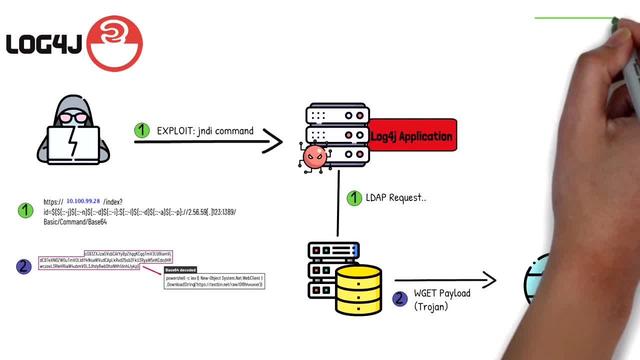 command that is targeting the vulnerable server. The second section is a shellcode that runs directly after the exploit, telling the machine what to do next after the exploit has gained access. In this case it's instructing the victim to download a Trojan using PowerShell. but we'll talk more about shellcode in the 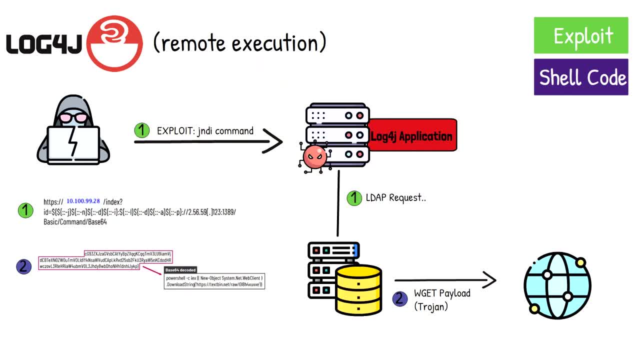 next section. This particular exploit may be referred to as remote execution and it comes from not properly sanitizing the input validation from the Java application. In this case, the actual exploit was the JNDI command you see on screen, which requests a malicious 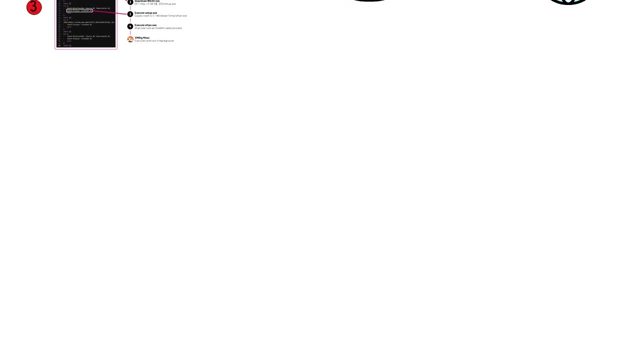 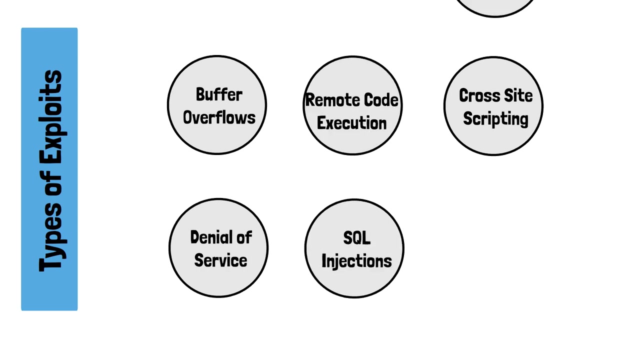 resource, which can be referred to as the payload. Many other kinds of exploits exist, depending on the intended purpose of the attack and the delivery mechanism, whether it's remote, local or client-based. Some of the other more common exploits include buffer overflows, remote execution, which we just saw, cross-site. 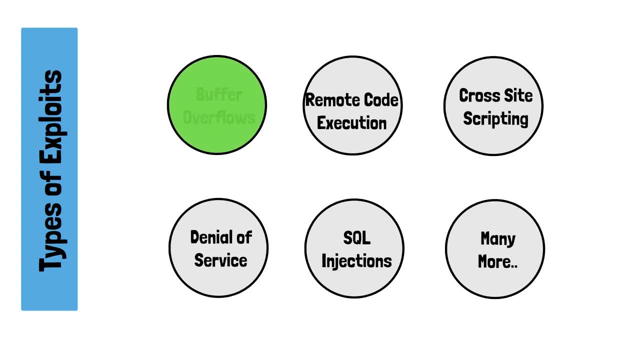 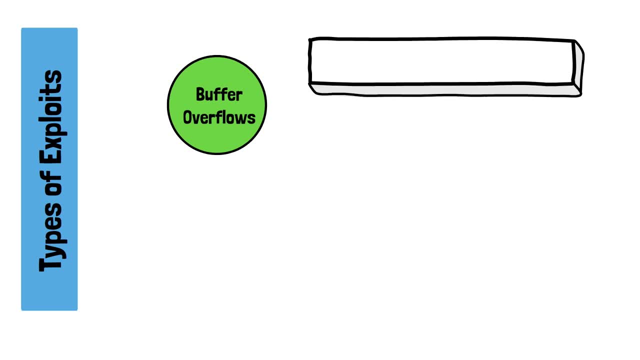 scripting, Denalo service, SQL injections and, of course, many others. One of the more popular exploit types is the buffer overflow. This type of attack varies greatly, based on many factors, but ultimately its goal is to introduce a system or kernel crash by overflowing. 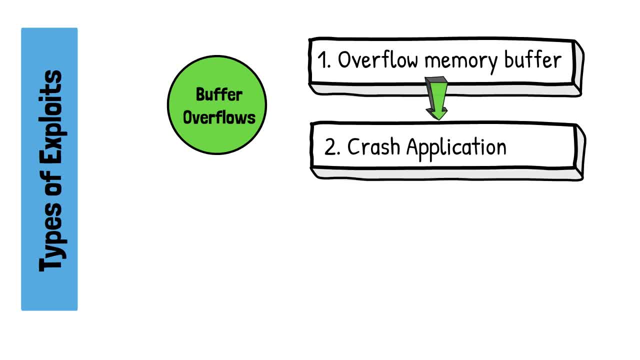 overflowing the memory buffer reserved for the application that is vulnerable. Once the application or system crashes, the goal is to insert malicious data in the memory buffer where the application was residing. From there, a common attack is to attempt to jump into a more privileged place in memory called jumping the stack. This is where the exploit points. 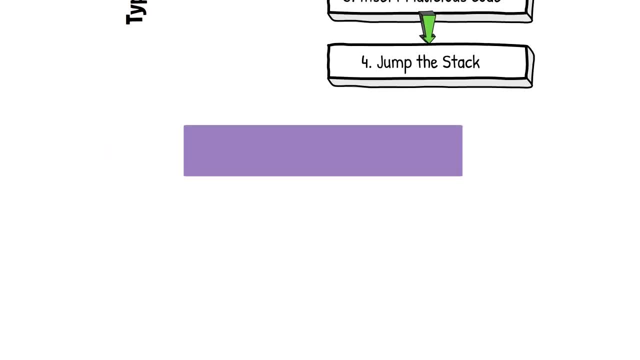 to shellcode, which contains machine-level instructions that we'll review in the next section. Let's look at a high-level example of a buffer overflow in action. Let's assume that an application has requested your username. The application has reserved 8 bytes of memory to store the username. An attacker that knows. 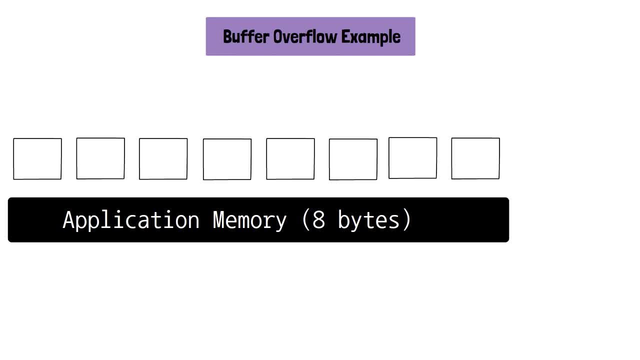 the input variable can only hold 8 bytes of memory, will attempt to overflow this buffer by inputting 10 bytes. These extra 2 bytes will then contain real code that can alter the execution of the program When the vulnerable application attempts to save this 10 byte. 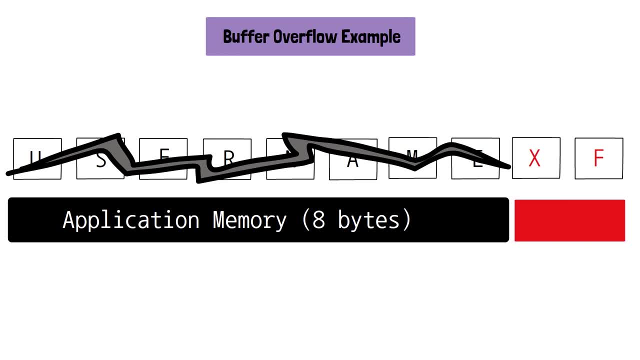 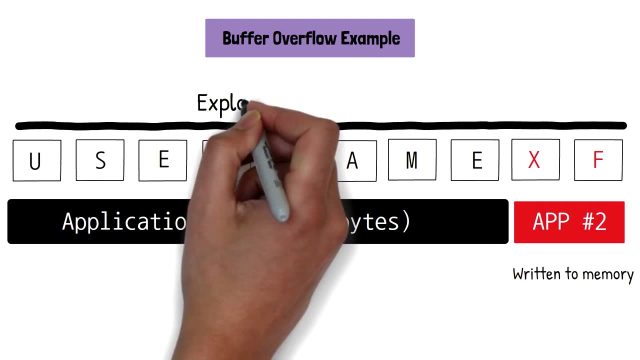 value, the application crashes and the two extra bytes are actually overwriting into another portion of memory. The overwritten part of memory now has these 2 bytes of real code that can then attempt to do other things, such as jump into a more privileged space in memory or run other kinds of shellcode. It's important to note that. 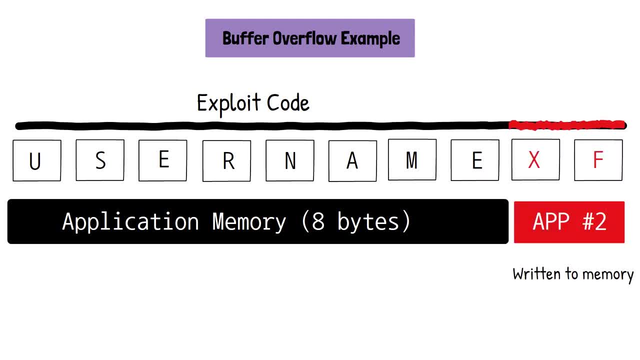 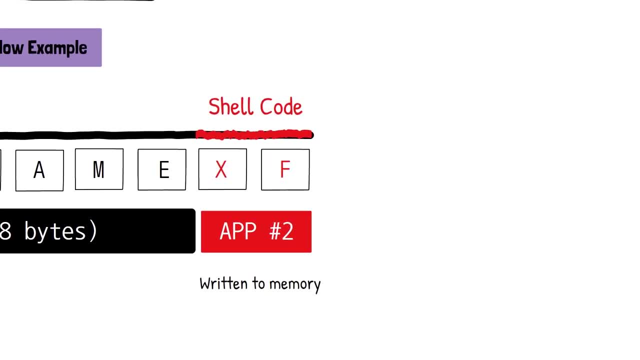 the buffer overflow is one of many types of exploit. In the buffer overflow example, the exploit inserts these 2 bytes of code into memory, which is used to execute the second part of the attack, which is a shellcode. The shellcode is typically written in assembly. 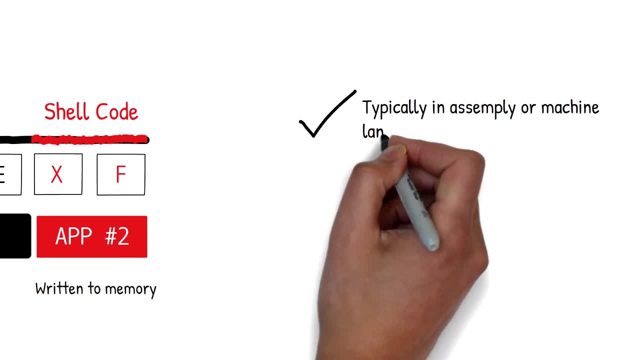 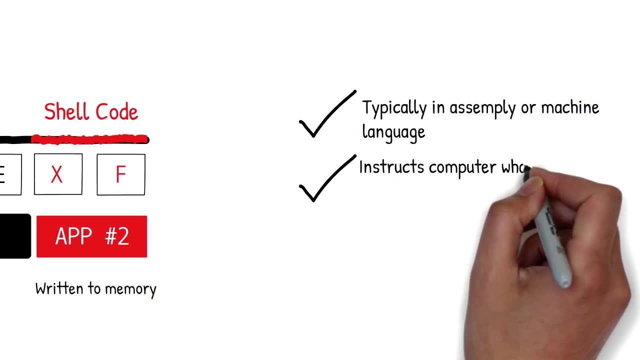 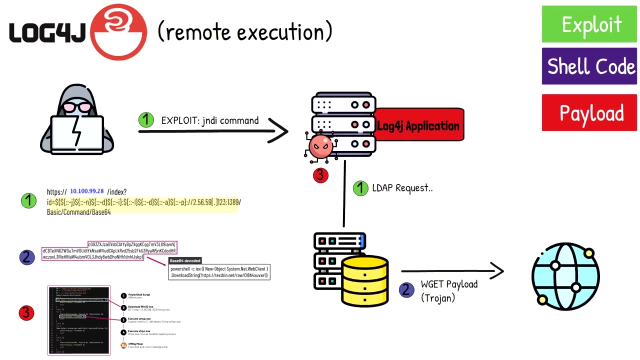 language because it involves memory, and it's a carefully crafted instruction that tells what to do at specific points of execution. Once a vulnerable system has been successfully exploited via buffer overflow or some other type of attack, the shellcode is the instruction that comes next. Going back to our log4j example, you'll notice that the code actually 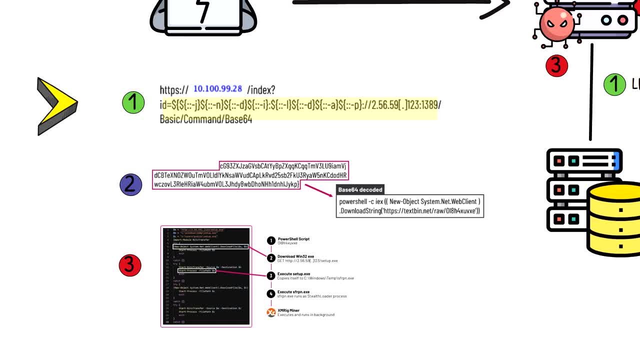 has these 2 parts: The first part, which is the exploit which we said earlier, is a JNDI remote execution command, and the second part, which is actually a powershell command which, translated from base64, means to download this malicious file from techspinnet. This first. 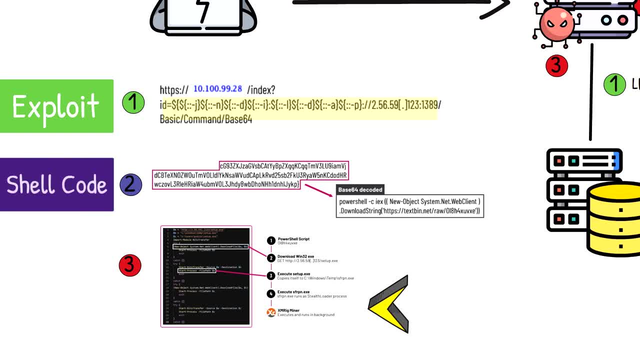 part is the exploit. The second part is the shell command which we want to run on the victim machine. Together, both parts make up a successful exploit. The shellcode is any type of payload that contains malicious code that you want to execute on the victim machine once the exploit has actually 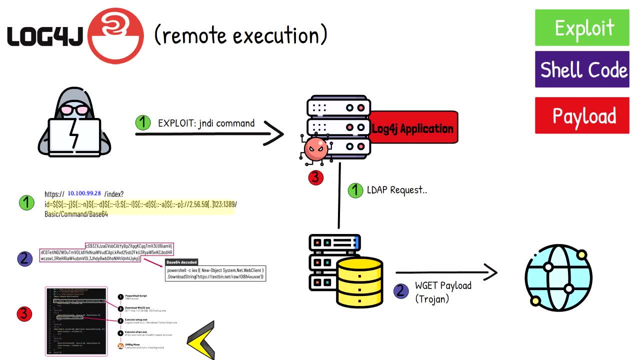 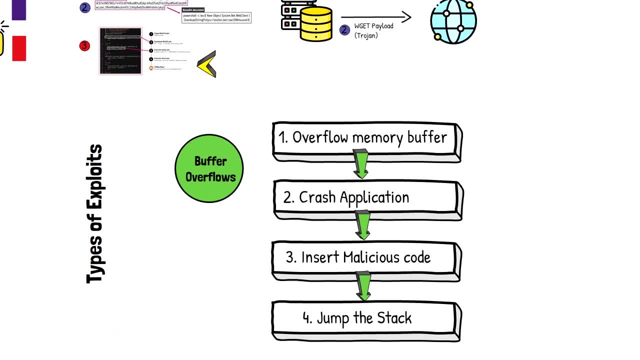 opened the door. Log4j was a rare example of a relatively simple type of exploit that had major ramifications. In this case, the shellcode is simple to understand because we're sending a remote command to be executed In more advanced exploits. things are rarely. 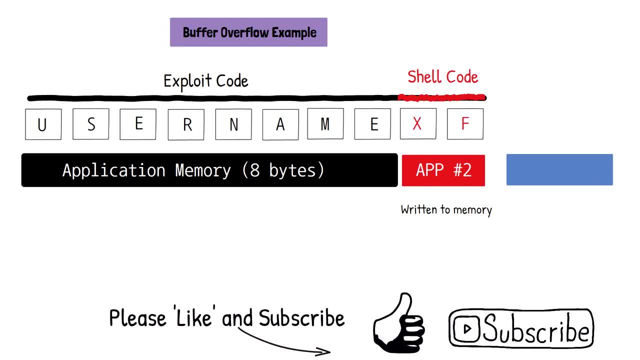 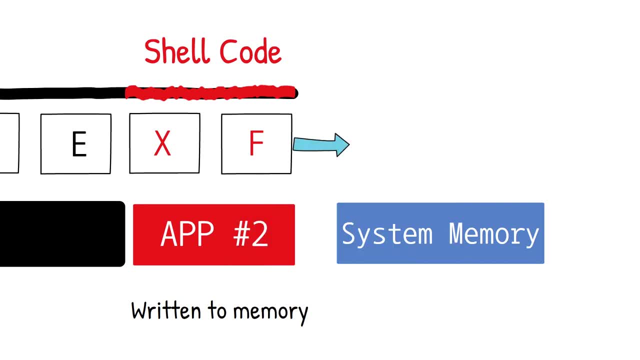 this easy. In fact, even in the simplest of buffer overflow examples, you rarely get to put your overflow code into the section of memory that is privileged to run the code that you want to execute. This is where jumping the stack techniques attempt to use pointers to redirect your code. 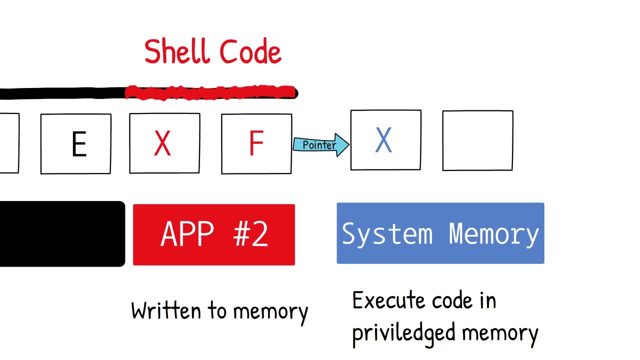 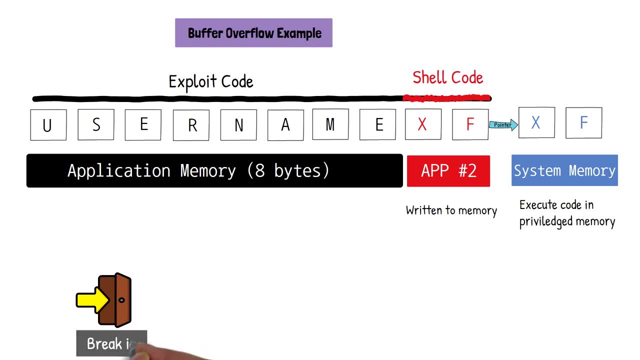 into more privileged sections of memory. While the shellcode can be considered a type of payload, this is a part of the exploit that is usually about doing just enough to get into the machine. Oftentimes, another type of payload is introduced as a third and possibly final step. that sets 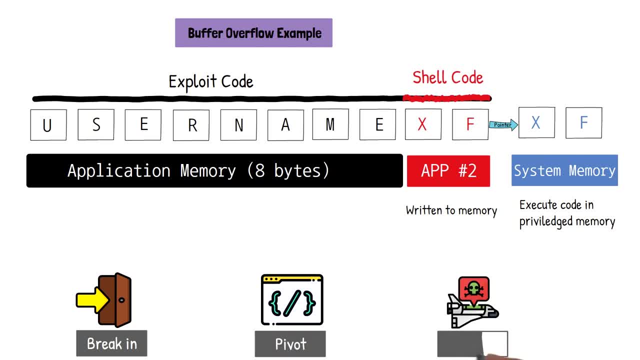 up an attacker with a more persistent entry to the vulnerable application. After a successful exploit, an attacker may opt to include another type of payload, which includes malware to carry out a specific attack, like a trojan, reverse shell or remote access tool. 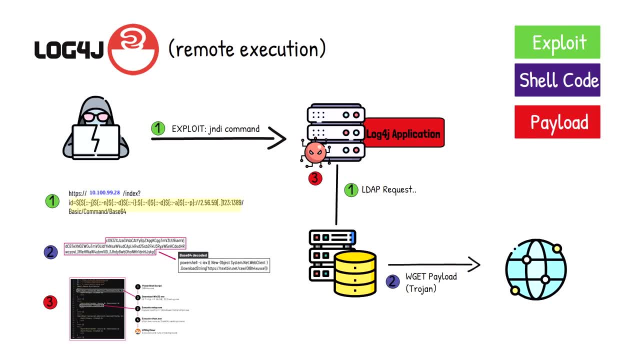 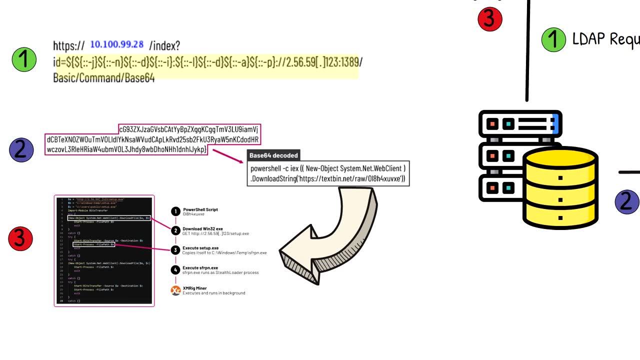 These can be used to gain further access later on. If we look again at our log4j exploit, we'll see that the shellcode actually triggers the download of a bit mining trojan. In this example, the trojan being downloaded is the payload and the final part of the successful 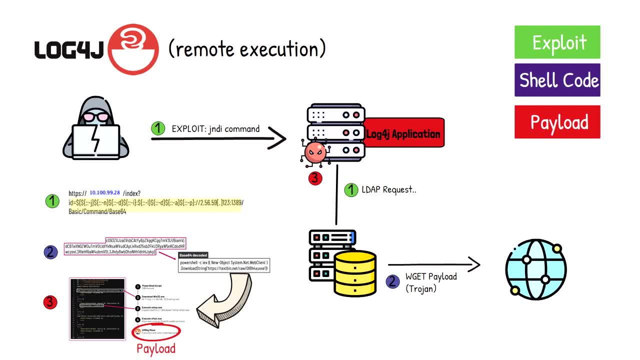 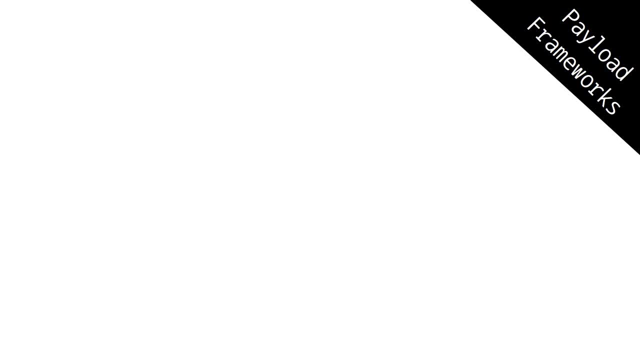 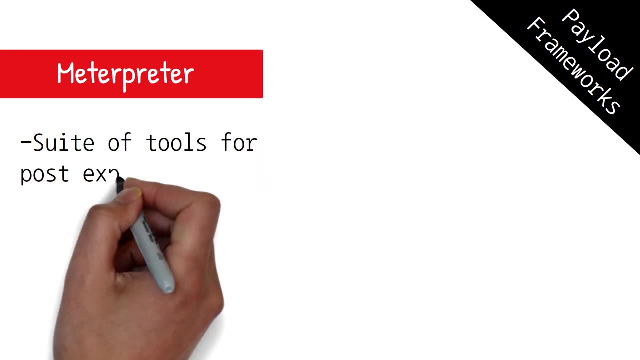 exploit because it accomplishes the goal of this particular attack, which is to run bit mining code on all infected systems. Several different frameworks exist for the kind of payload we want to run on the victim machine once the exploit has gained us access. Meterpreter is one kind of payload that itself includes a suite of tools that an attacker 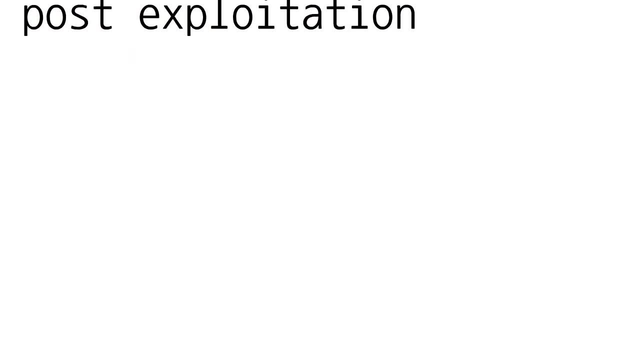 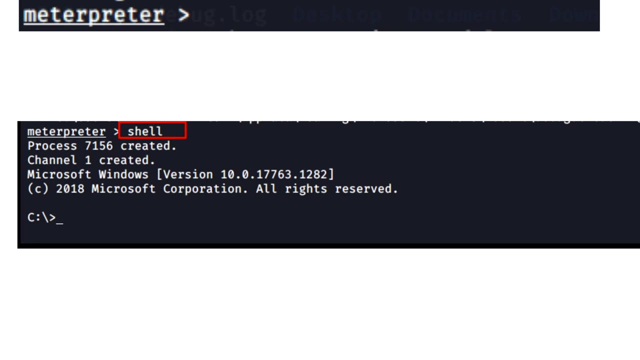 can commonly use on the compromised machine. With the meterpreter payload injected after the exploit, an attacker can do things like retrieve hash jumps from the SAM database, escalate privileges, turn on and use webcam features, drop into the shell prompt, automatically cover up the tracks, which removes logs. that 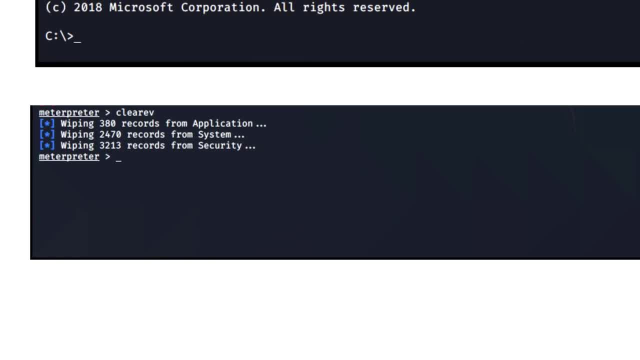 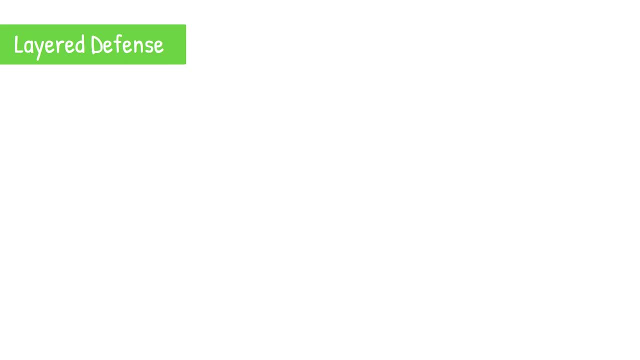 may have been triggered during the compromise and many other functions. Several free and commercial tools exist to protect against most of the techniques that we've discovered in this video, But like all things in security, nothing is a silver bullet and a multi-tiered defensive. 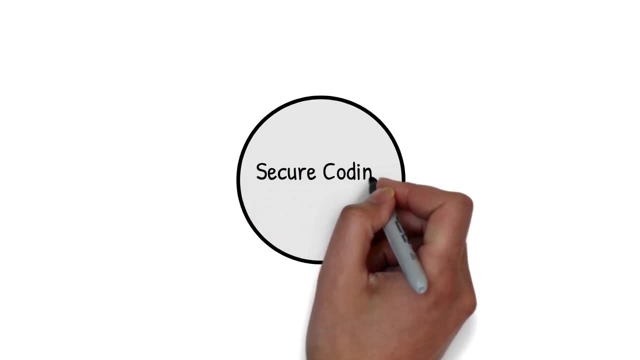 approach is necessary. It starts with secure coding of the application- There's a lot of information about the application or software- and making sure that proper security practices are in place during the time of development. Several great resources exist from Microsoft, OWASP and others that provide the developers.